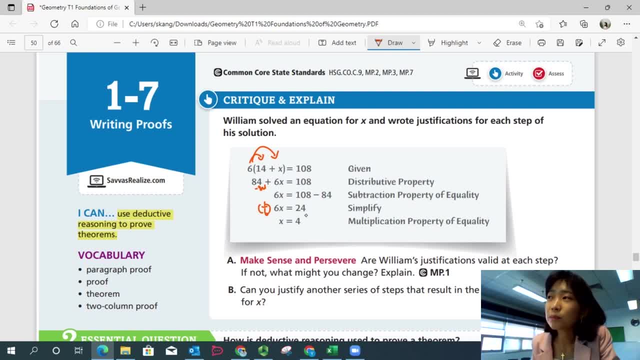 But that also means that we can divide both sides By 6.. This could also be a multiplication property. Instead of multiplication, this could also be a division property of equality, If he divided each side by 6, instead of multiplying by a fraction. 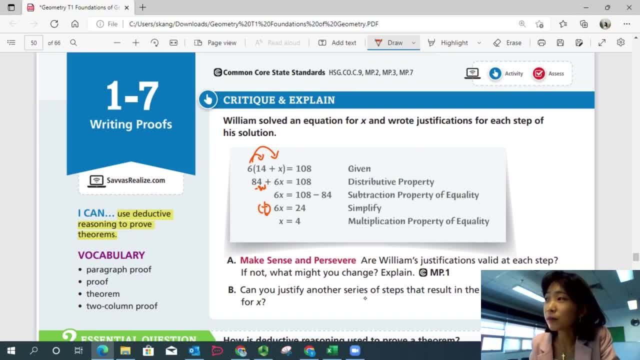 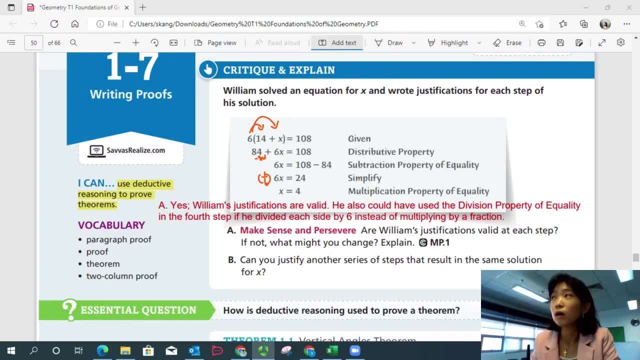 Okay, So can you justify another series of steps that result in the same solution for x? So we can try to solve this in different ways, But we're going to start with the given information: 6 times 14 plus x equals 108, and that's given. 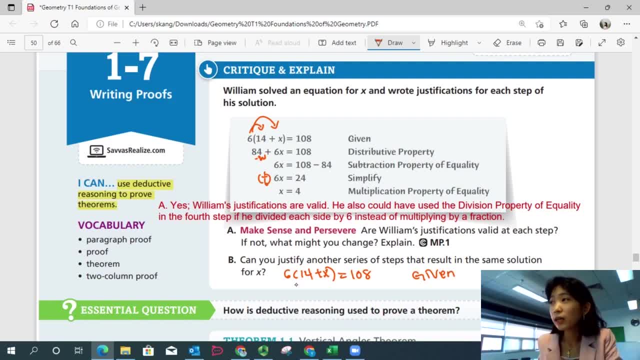 How could we go next? Instead of using distributive property, what else could we do? How to like? what is another way to solve this? You can divide both sides by 6, so that we have 14 plus x here. 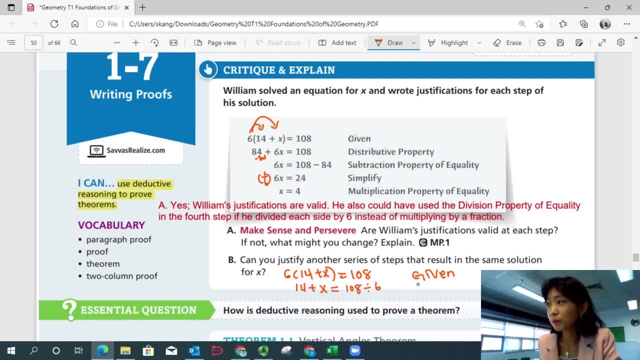 We have 108 divided by 6. And that's division, property of equality. And then we can simplify and get 18.. And then we subtract 14 on both sides and have x is equal to 18 minus 14.. And that's a subtraction. 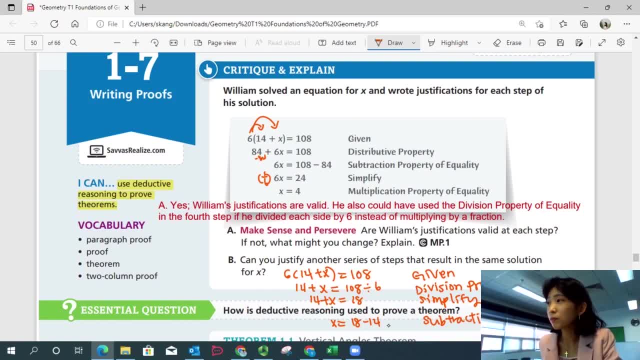 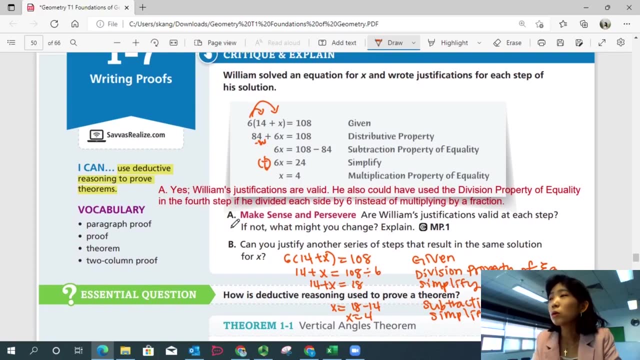 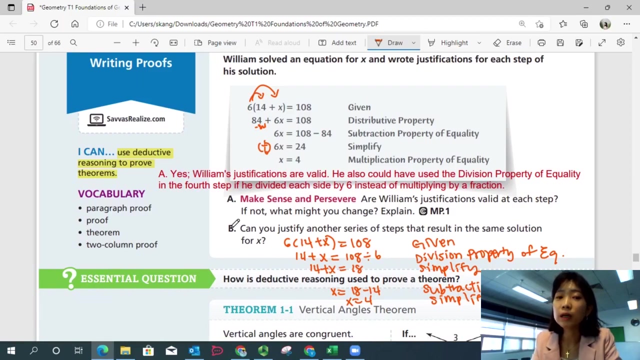 So we have: x is equal to 4.. You should get the same answer. Okay, So there are multiple ways, different ways to solve the same kind of problem, But the answer must be the same. So let's think about this essential question. 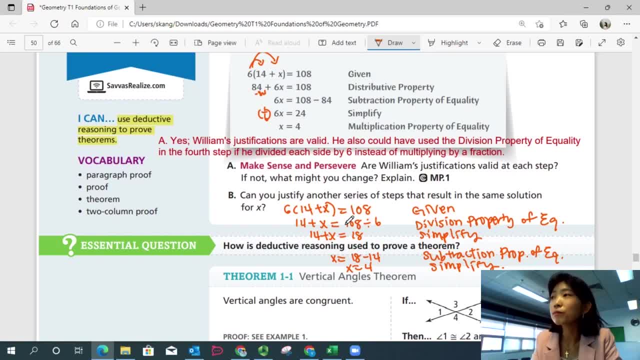 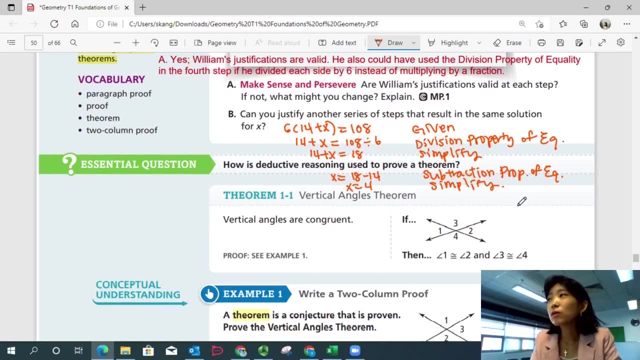 How is deductive reasoning used to prove a theorem? We have a theorem 1-1, vertical angles theorem. So vertical angles are congruent. is what this theorem is saying. We're going to have to prove this before we use them. 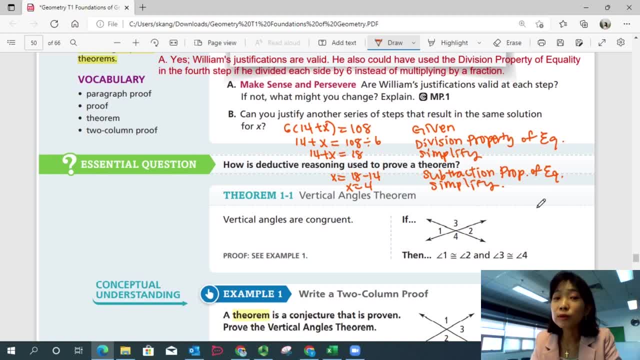 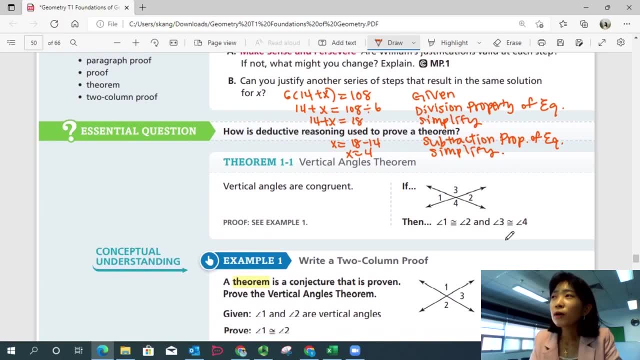 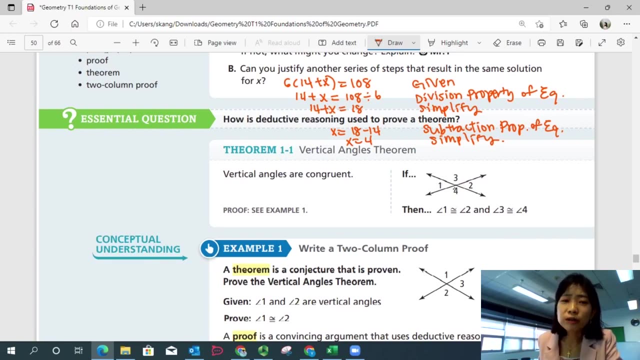 Theorems are not proven until we prove them, But theorems could be proven, Okay, So we're going to prove that in example 1.. First of all, what are vertical angles? Vertical angles are angles that are vertical to each other. 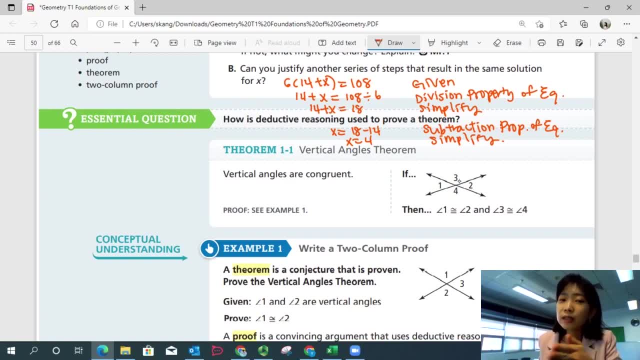 So they're not right next to each other, They're not adjacent angles, But they're the angles on the other side of the intersection. Okay, So if you have four angles formed by these two lines, then angles 1 and 2 are congruent and 3 and 4 are congruent. 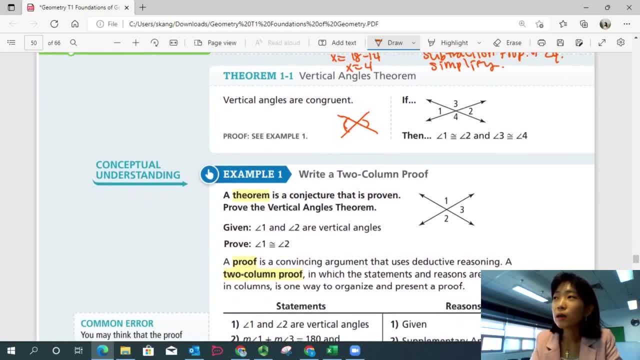 So let's prove this. First of all, what is a theorem? A theorem is a conjecture that is proven. Prove the vertical angles theorem. It's already proven And so let's prove it together so that we can also use this theorem in the future to prove other theorems. 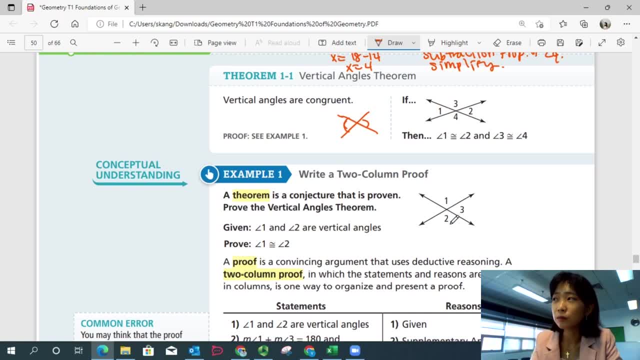 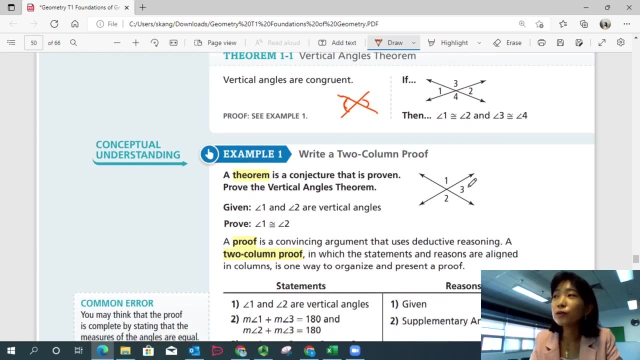 So it's given that 1 and 2 are vertical angles, We're going to prove that they're congruent, And a proof is a convincing argument that uses deducted reasoning, using facts. A two-column proof in which the statements and reasons are aligned in columns: 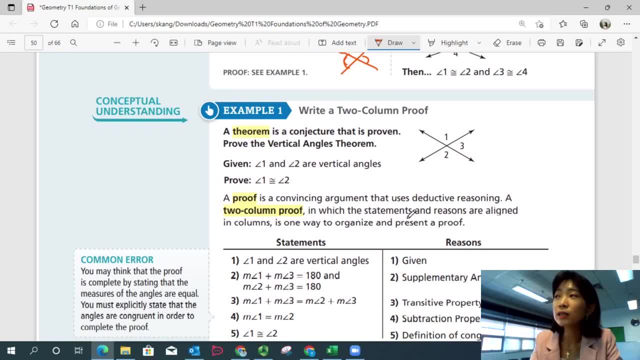 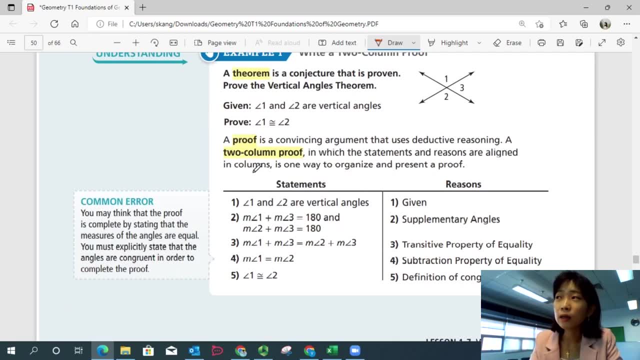 is one way to organize and present a proof. This is the first type of proof that we're going to look at. Two-column proof: You have two columns, with the first column being the statements and the second column listing the reasons. Okay, Very obvious. 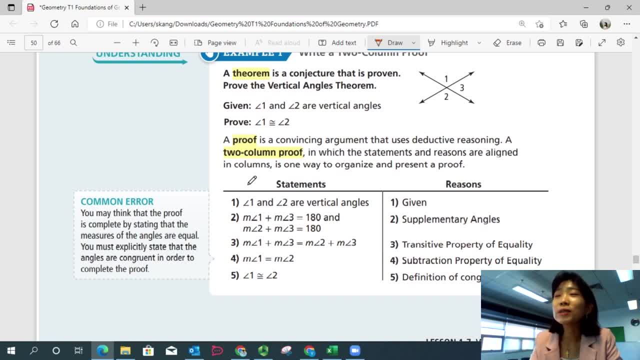 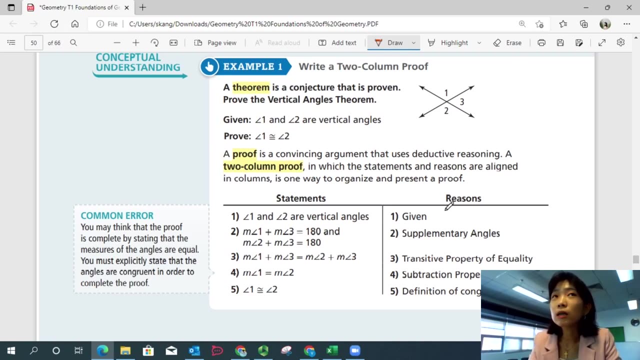 And it's very clear. Okay, So the first type is almost always going to be a given fact. We're going to start with given: Okay, Angles 1 and 2 are vertical angles. It's the given fact. And then what can we conclude from that given fact? 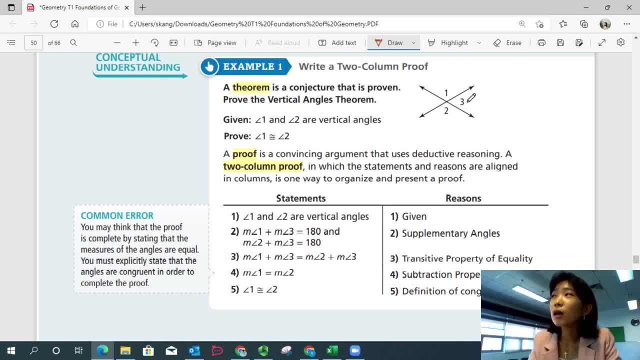 Before we do that, what are other angles that we could use? So if we have an angle between 1 and 2, angle 3.. Angles 1 and 3 make a line. Angles 2 and 3 make a line. 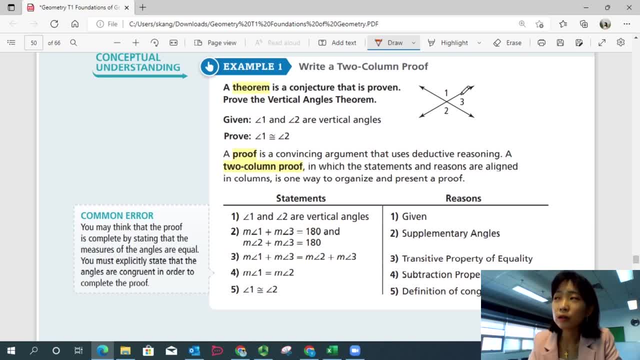 So the sum of those angles should be 180. By the definition of supplementary angles. Okay, Using this information, where are we going? Because measure of angle 1 plus 3 is 180.. And 2 and 3 make a supplementary angle as well. 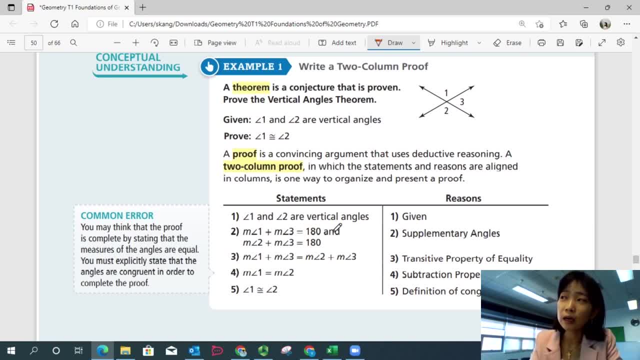 They're both going to be 180 degrees when they're added up together. So we're going to make those statements equal to each other. So measure of angle 1 plus 3 is equal to measure of angle 2 and 3.. 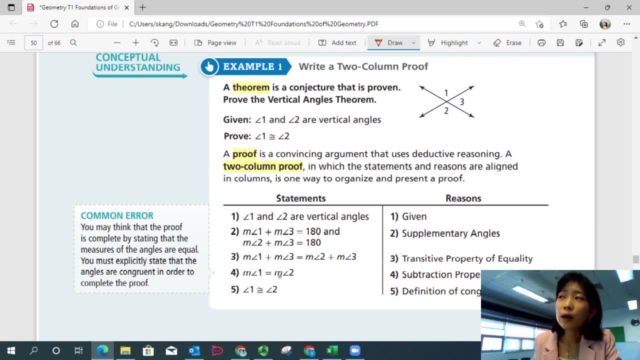 Right. So then, solving for the equation, simplifying it, we can subtract measure of angle 3 on both sides, because it must be the same angle Right, And so that means measure of angle 1 and 2 must be the same. 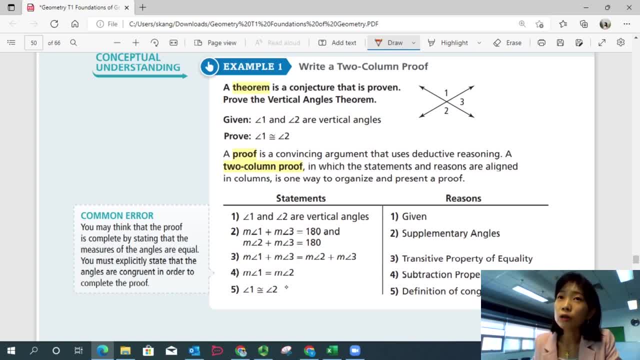 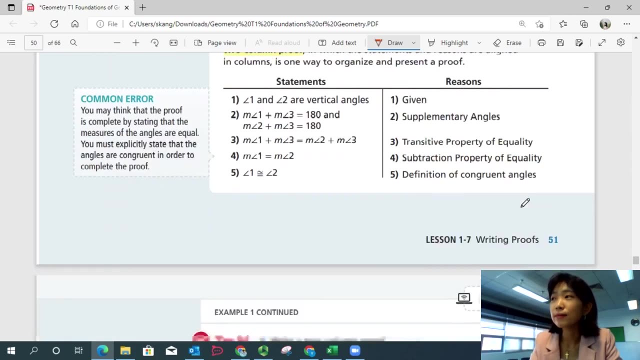 which makes, by definition, the angles congruent. Okay, So now we have proven with the two-column proof that vertical angles are congruent. Any vertical angles given would be congruent. All right, Now it's your turn. Try number 1.. 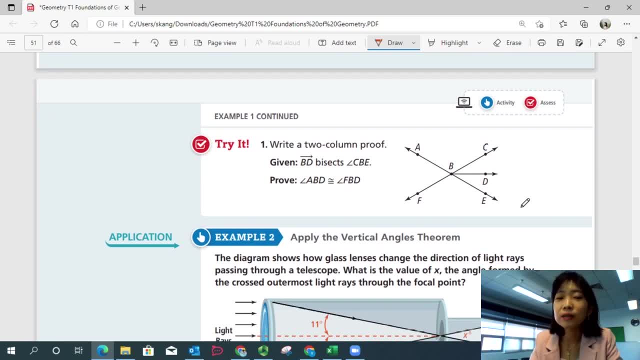 Write a two-column proof by yourself. See if you can try by yourself. With a given fact that the ray BD bisecting angle CBD, what are the facts that you know? What are the definitions that you know already In order to help you prove that angle? 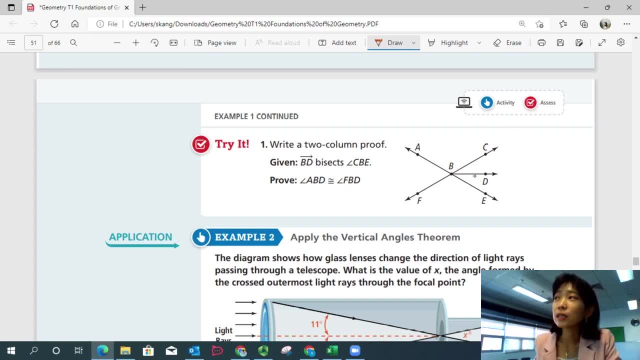 ABD is congruent to angle FBD. All right, Pause the video. Come back when you're ready for answers. Okay, Are you ready? Yeah, What do you do? First of all, you need to write two columns. Okay, 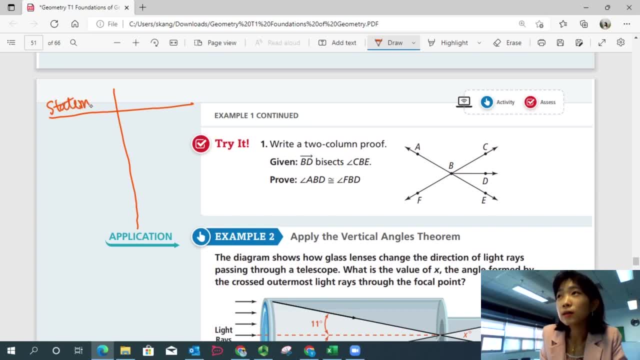 So the first column would be statements, The second column would be reasons, And then you will start with the given information: Ray BD bisects angle CBE, And the reason is that it's given. And then what do we know about an angle bisector? 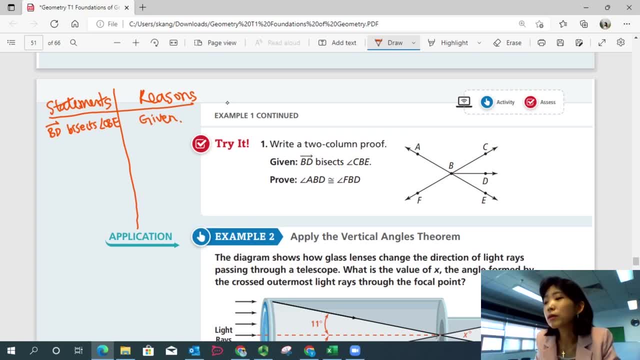 You divide the angle in exactly half Right. So that means this angle and that angle should be the same Right. They're congruent. So angle CBD is congruent to angle EBD. What is the reason? This is by the definition of angle bisector. 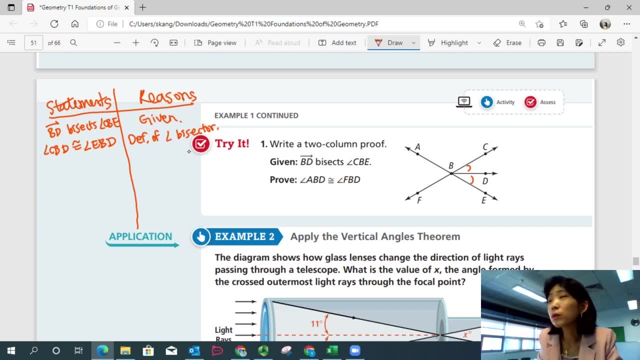 Okay, And then what do we just learn about? vertical angles ABC and FBE should also be congruent because they're vertical angles, Right? So angles ABC and FBE are congruent by the definition of vertical. Oh wait, 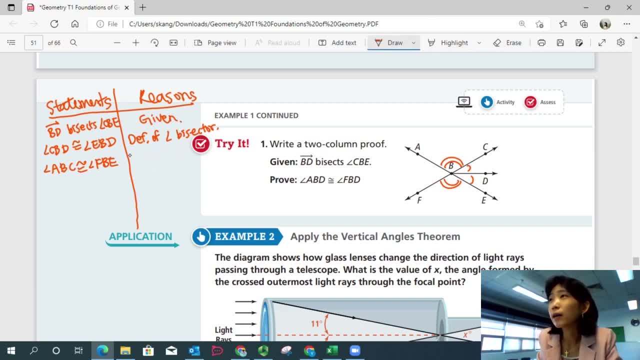 This is not a definition. Sorry, You can say by vertical angles theorem. Okay, I'm abbreviating them, But this is vertical angles theorem. What's the next step Now, using these two facts that we concluded using deductive reasoning? 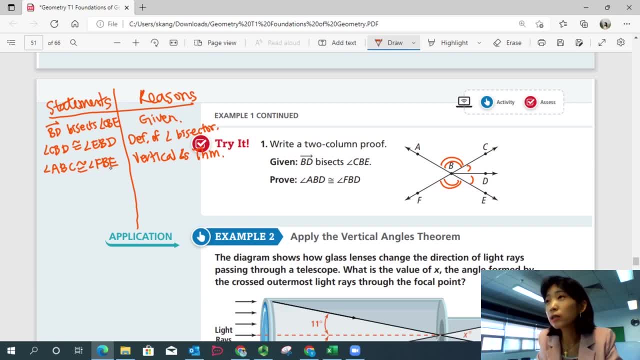 we're going to use angle addition postulate so that what is ABD ABD is angle ABC and CBD combined together, added together, Right, We're going to add these two to get angle ABD. Add these two to get angle FBD. 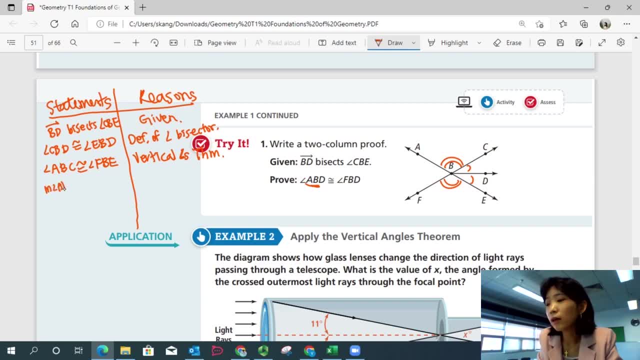 Okay, So measure of angle ABD is equal to measure of angle ABC plus measure of angle CBD. And measure of angle FBD should equal to measure of angle FBE plus measure of angle EBD. And what is the reason? By angle addition postulate. 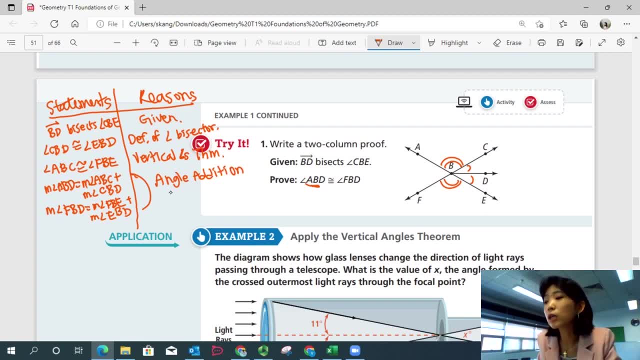 So you are using all the postulates and theorems that you have already learned previously. But if you know something that you didn't learn yet, you have to go. in geometry, the order is really important. So if you haven't proven it before, we haven't talked about it, then you cannot use it. 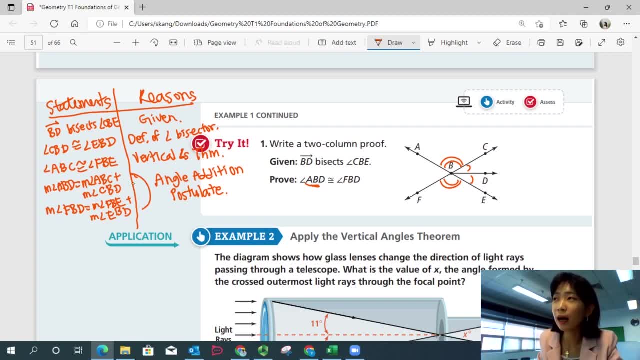 you cannot use it. okay, so make sure that we have gone over the postulates and the theorems in the past before you use it. so every, every time we learn a new theorem and new postulate, you should be excited about it, because there are more things that you could use to prove. 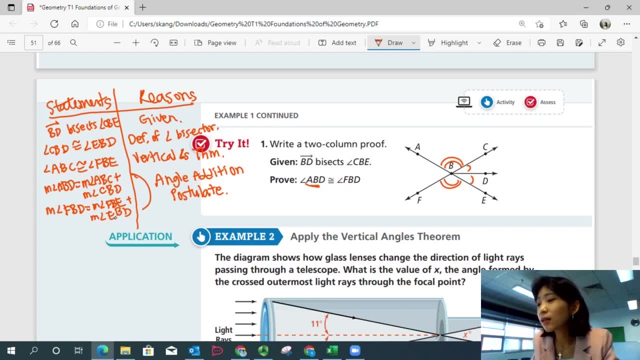 all right, um, the next step now. we know that, um, um, looking at this, how can we, how can we, uh, combine these together? because remember that we're trying to prove that these two angles are the same, right, so, because they're equal to each other, and they are equal to each other, and we know that angles a, b, c and f b e are congruent. 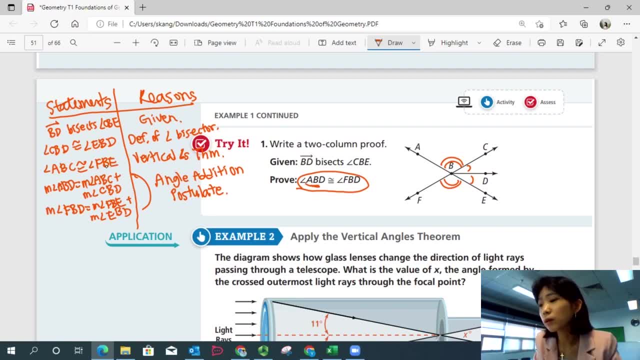 we substitute either one of them right and say measure of angle a b d should be the same as adding measure of angle f b e instead of a b c. notice that substitution plus measure of angle e b d. okay, so by substitution property of equality, we substituted. 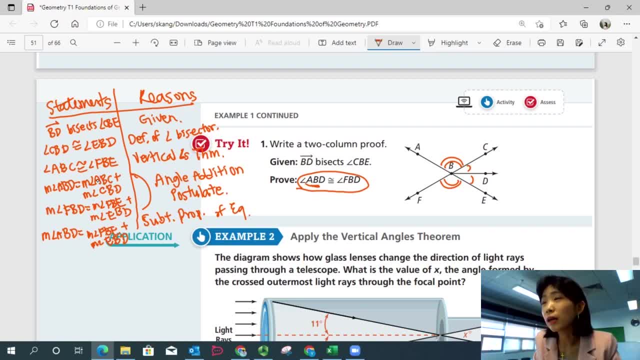 f b e instead of a b c. okay, and then you can say that, oh, the measure of angle a b d is equal to measure of angle f b d. why can't we just skip step, uh, and then say, oh yeah, it's. it's obvious that we can make them equal to each other. we need a middle step to to prove them and provide real 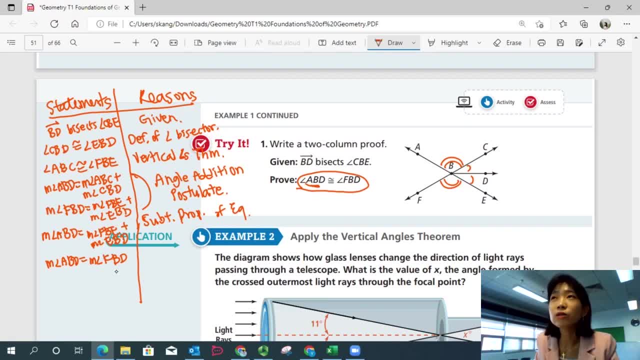 reasons about it. okay, you can't just skip steps. try to try to write down as many steps as possible so that you're very clear. okay, you can't just, you know, start from a given and then you can say, oh yeah, because of this, there that theorem, uh, you can prove that. 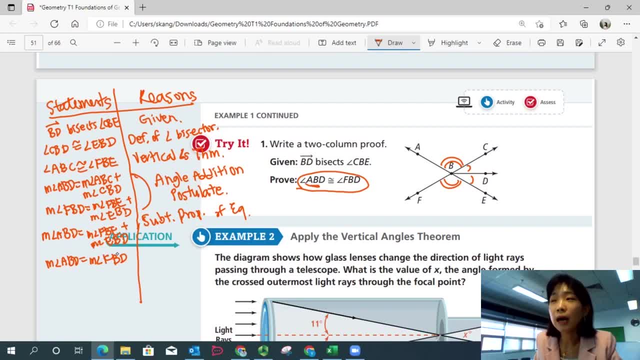 this is correct. you have to write down the whole steps, okay. you have to show them thoroughly, okay. and then: uh, yeah, this is because of the transitive property of equality. remember, if a equals b and b equals c, then a equals c. that is called the transitive property. 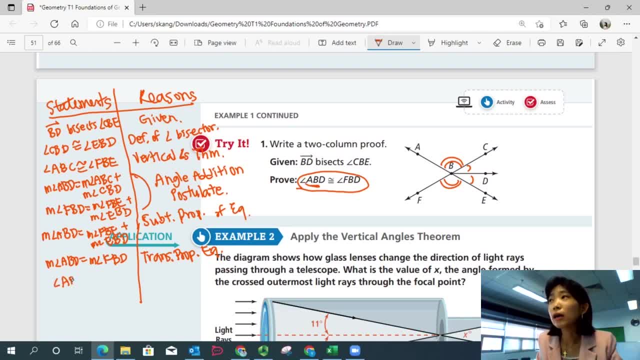 so finally, you can say angle a b d is congruent to angle f b d, because the measures are the same and that's the definition of concurrent angles. okay, seeing we can't say anything else, one more thing, yeah, um, they say this can be an advantage. 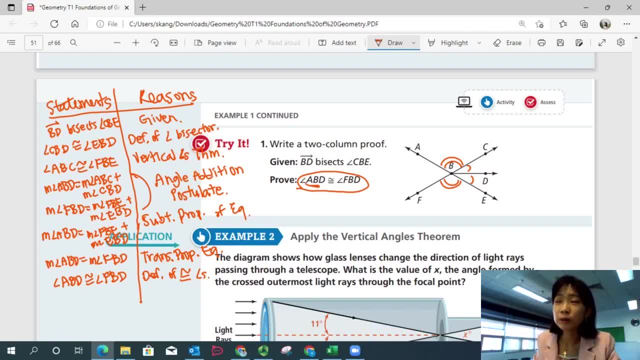 so our um, this can make us fool it. attempt exactly how long was. yeah, that was a long triad question, but, um, I hope you got it. if you proof, So we've done great. So you can keep practicing writing a two-column proof to get. 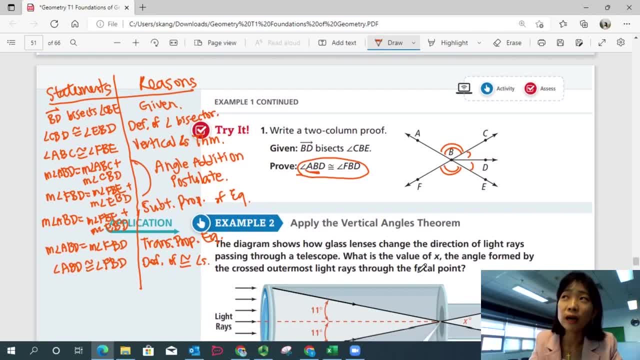 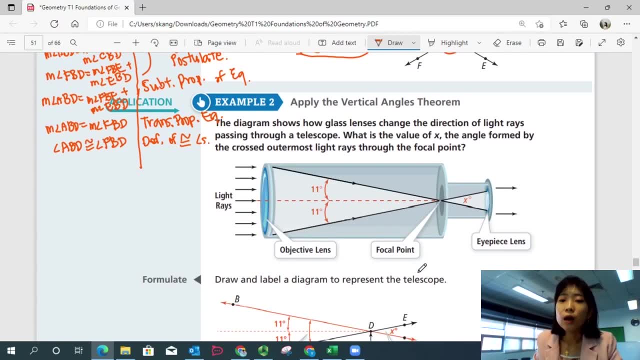 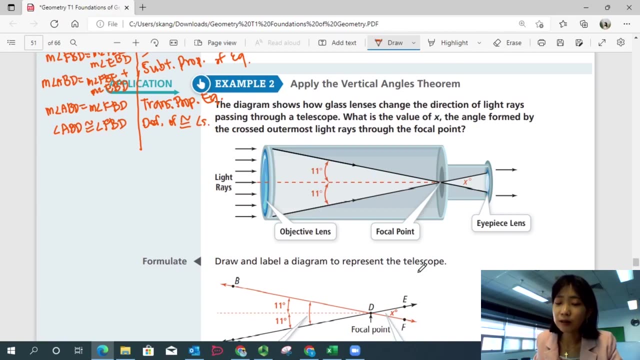 better and better. Just make sure that you write every step and write all the reasons down for each step. Justify, All right. let's look at example two. Apply the vertical angles theorem. The diagram shows how glass lenses change the direction of light rays passing through a telescope. 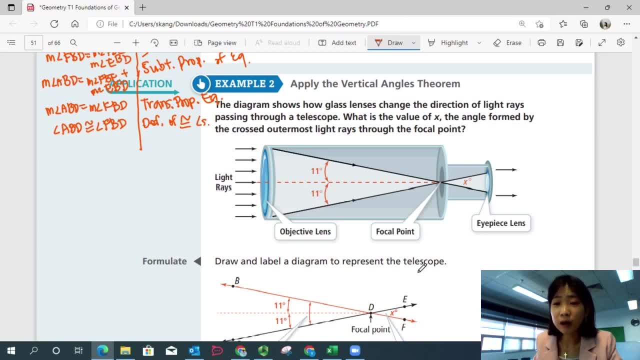 What is the value of x? the angle formed by the crossed outermost light rays through the focal point. So we see a light rays going through here And then this is the objective lens that it's going to go through. We see a focal point and the light rays are going to go perpendicular. 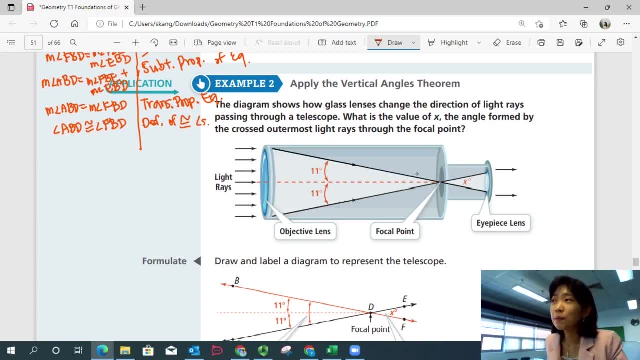 through this lens And it's going to bisect the angle. So we have an angle from the focal point to objective lens. You see that 11 degrees, And we have eyepiece lens on the other side. So we want to figure out the x which will. 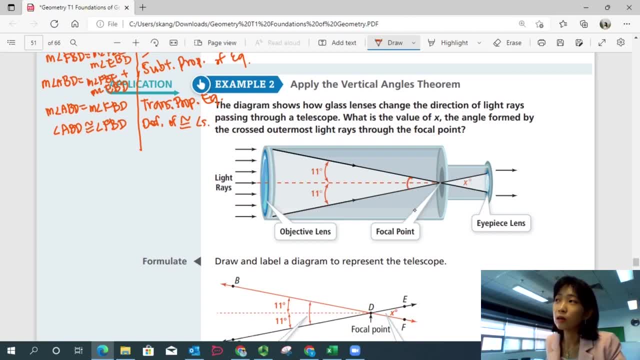 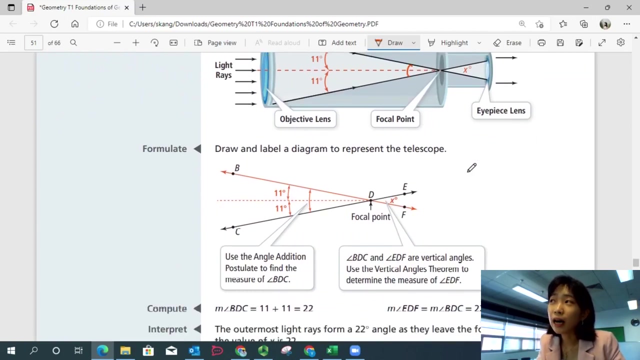 be the vertical angle to this angle, which will be addition of these two angles. So just by looking at it you can say you can figure it out right, It's going to be x, It's going to be x, It's going to be 11 plus 11, 22.. But can you reason that out? You can draw and label. 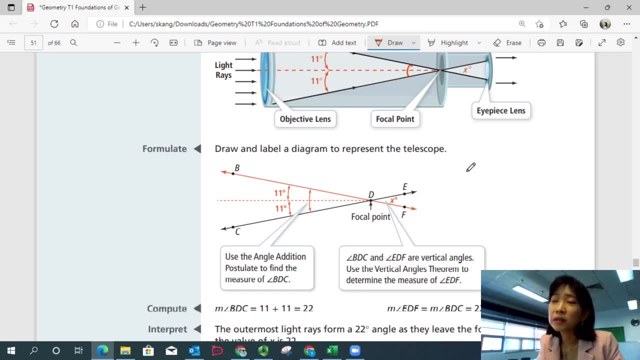 a diagram to represent a telescope. How do you know the vertical angles? How do you reason that out? You can use angle addition postulate to find a measure of angle BDC, which is 22. And BDC and EDF are vertical angles. 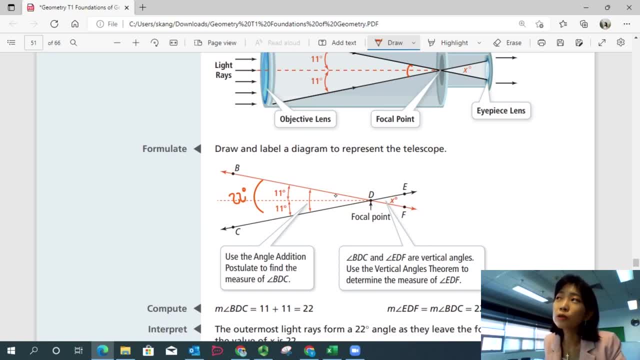 So what we have here is a vertical angle. If you look at the x-axis, you can see that these angles are very similar And the vertical angles are very similar. The vertical angles are. So if you look at the x-axis, you can see that the x-axis is very similar to the vertical. 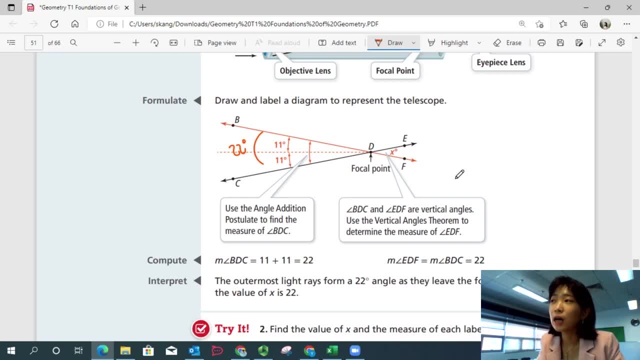 angle. So you can use the vertical angle theorem to determine that angle x is also going to be 22 degrees. So the outermost light rays form a 22 angle as they leave the focal point. So the value of x is 22 is our answer. 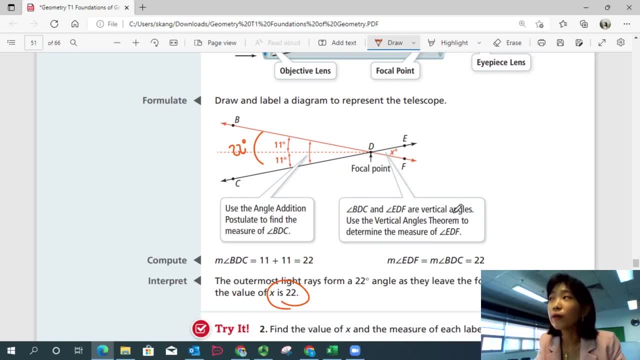 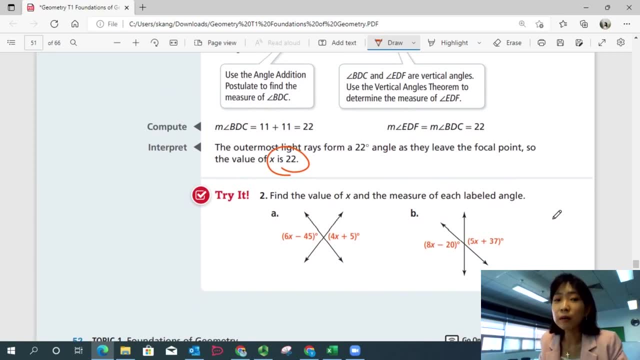 Okay, so use the x-axis. You can use the theorem to figure out algebra in real life as well. Try number two: Find the value of x and the measure of each labeled angle. See if you can figure out x and then figure out the angles by yourself. 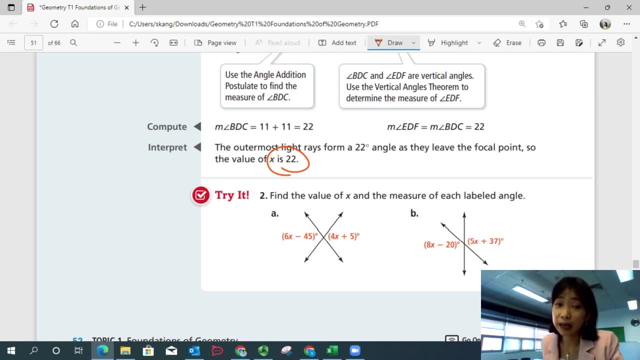 Make sure you're not stopping when you figure out the x. x is not the angle. You need to figure out the angle after you figure out x. Okay, come back when you're ready for answers. Are you ready, All right? part A: 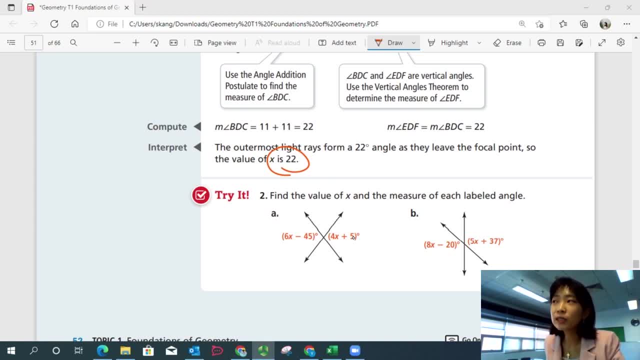 They're vertical angles and they have different expressions, but you can set them equal to each other. 6x minus 45 should equal to 40x plus 5, because they're vertical angles. Vertical angles have the same measure of their angles, right. 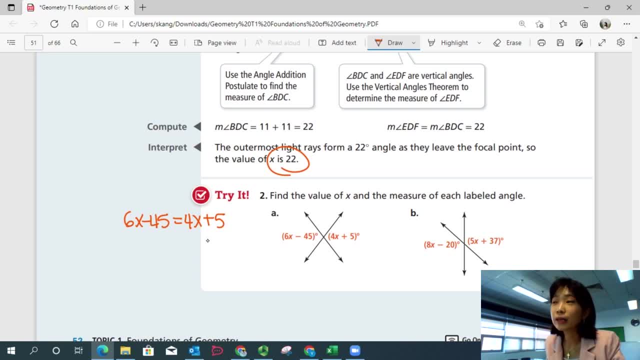 So now it's a matter of solving for x. Simplify, simplify and solve for x. So add the like terms. We don't have like terms in either of the sides, so what do you do? You have to subtract some terms. 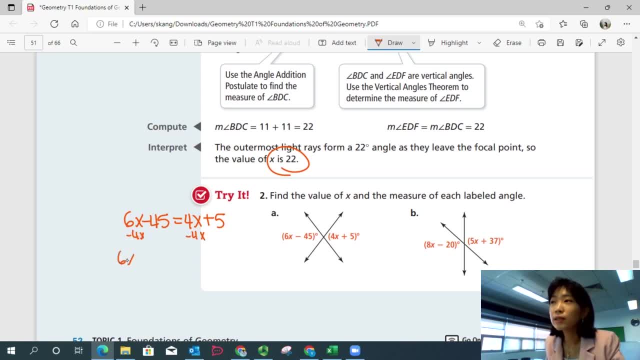 Subtract 4x on both sides. So then you have 6x minus 4x and add 45 on both sides And that's equal to 5 plus 45.. So 6 minus 4 is 2x, 5 plus 45 is 50. 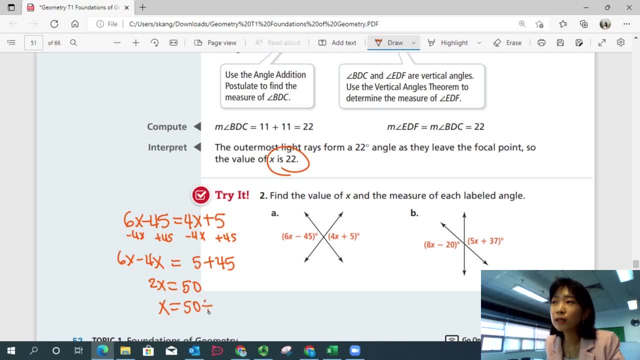 X is equal to 50 divided by 2.. If you divide 2 on both sides, so that's 25.. Are you done? No, Because x is 25, you can figure out the angle by plugging in 25 into any of these expressions. 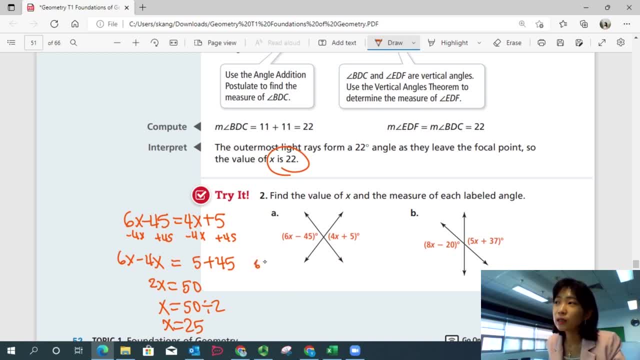 You're going to get the same number. What do you get? 6 times 25 minus 45, or 4 times 25 plus 5 is going to give you 105.. Okay, So, first of all, your x is 25, is your answer. 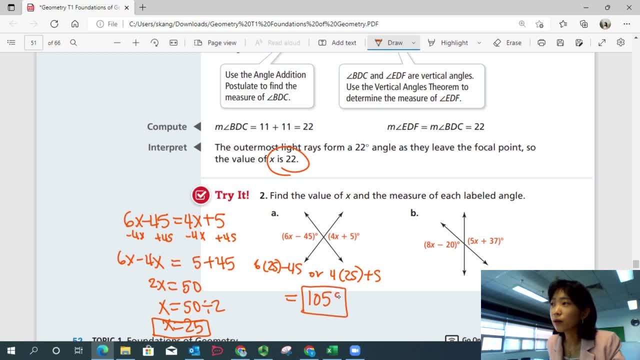 And then the angle. Angle is 105 degrees. It's another. your next answer. What about part B? What is your x? So setting up the equation: 8x minus 20 is equal to 5x plus 37. You do the same thing. 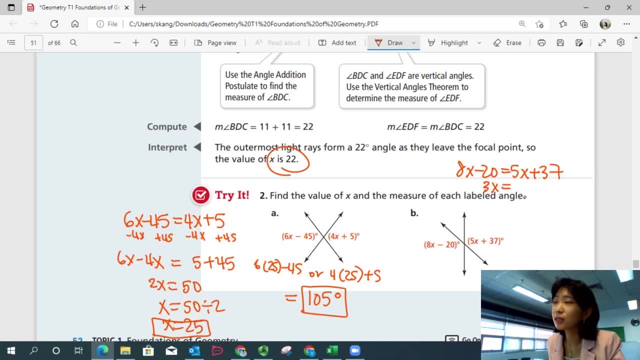 Subtract 5x: 5x on both sides, you get 3x. Add 20 on both sides, you get 57. And x is 57 divided by 3, you get 19.. So x is 19, is your first answer. 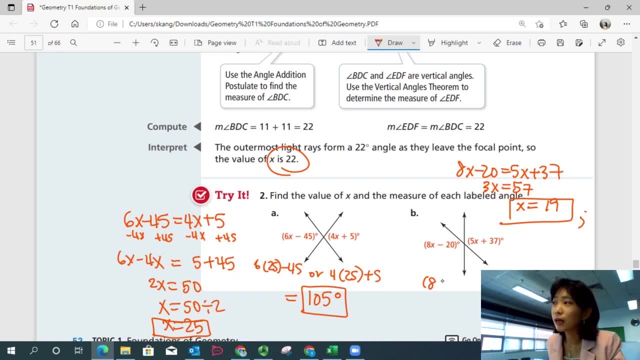 If you plug 19 into your equation, 8 times 19 minus 20, or 5 times 19 plus 37,, will give you 100. And 32 degrees. Okay, Check your answers. You got both of them correct. 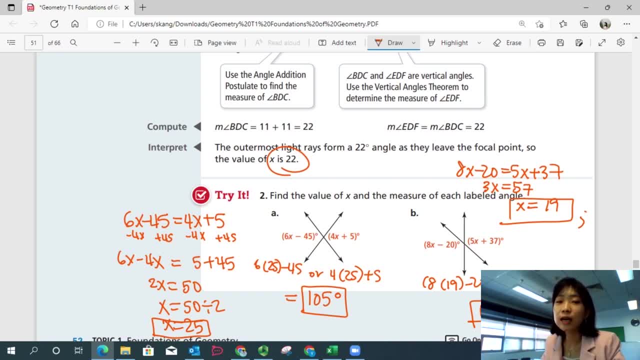 Good job. You figured out the x's and you didn't figure out the angles. Try again, See if you can get it. Make sure you solve for the angles, Alright, Next theorem 1-2.. Congruence Subtract. 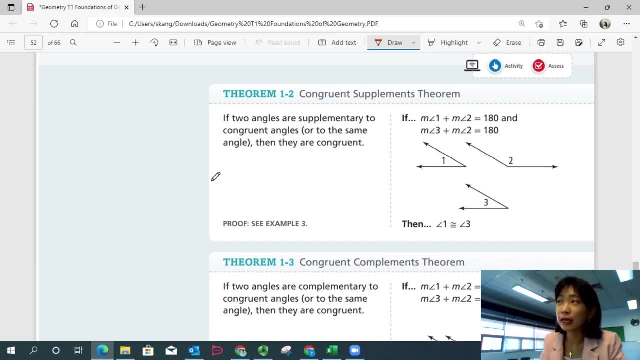 If two angles are supplementary to congruent angles or to the same angle, then they are congruent. Okay, What are supplementary angles? They are supplementary. They make 180 degrees when they are added together. So if measure of angle 1 and 2 is equal to 180,. 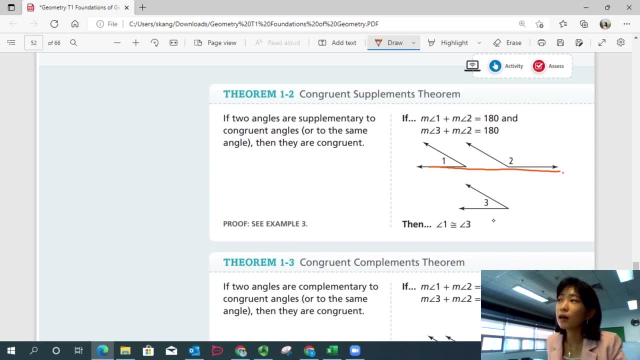 then this should be a straight line. And if measure of angle 3 is equal to 180, then they should also make a straight line. But angle 2 should be the same. So that means there is only one supplementary angle that is supplementary to angle 2.. 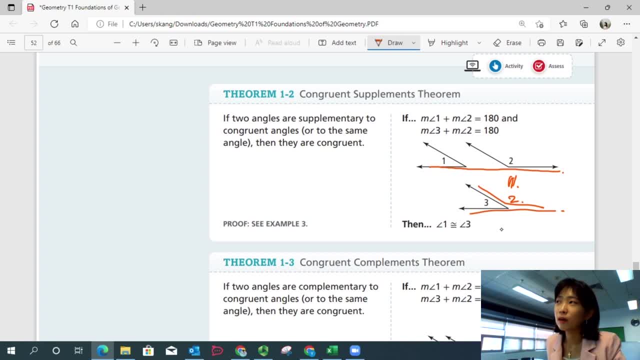 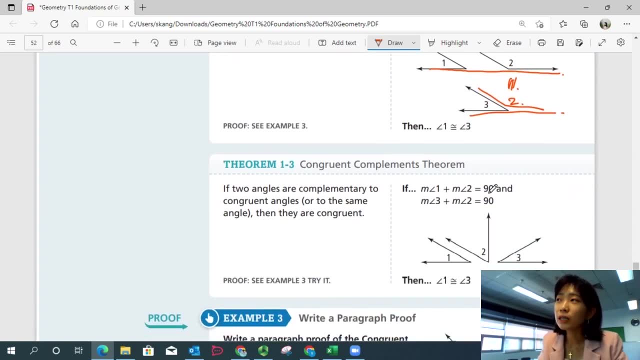 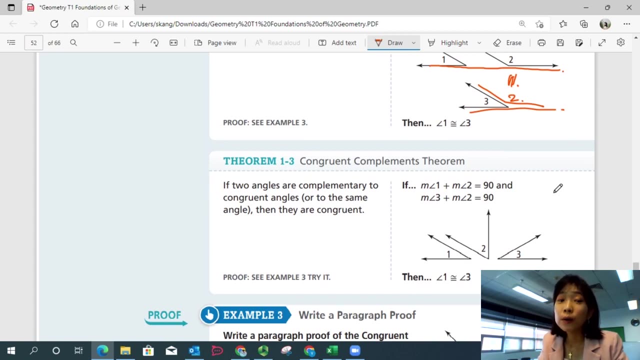 So angles 1 and 3 must be the same. Okay, We're going to prove that in example 3.. Theorem 1-3.. Another one Congruent complement theorem: What is a complementary angle When those two angles add up? 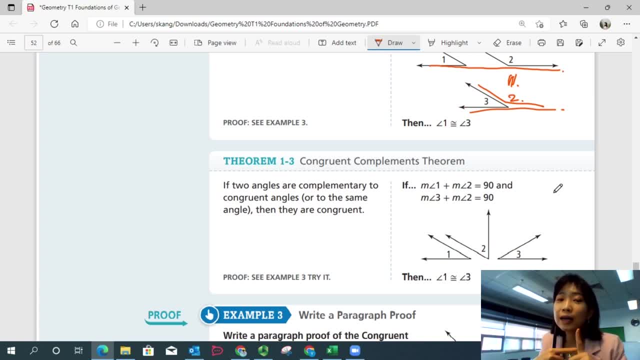 they don't make 180 degrees, They make a 90 degree. So this is supplementary, This is complementary. Okay, Supplementary angle is 180.. Complementary angle is 90 degrees. Okay, So the theorem says if two angles are complementary to the same angle, 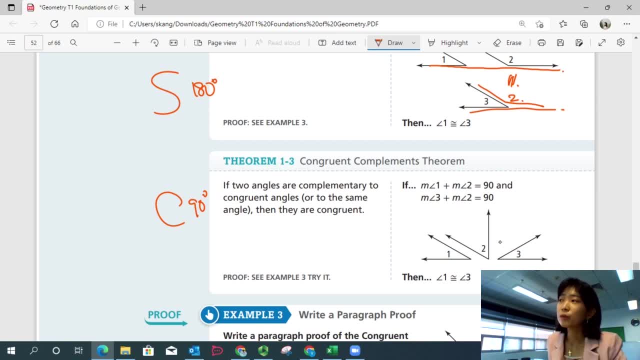 then they're congruent. Okay, Because in the same reasoning there is only one angle that could be a complementary angle to the same angle. So if they're complementary to the same angle, then they must have the same measurement and they're congruent. 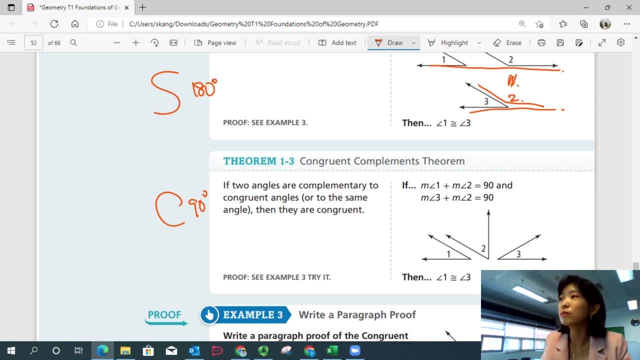 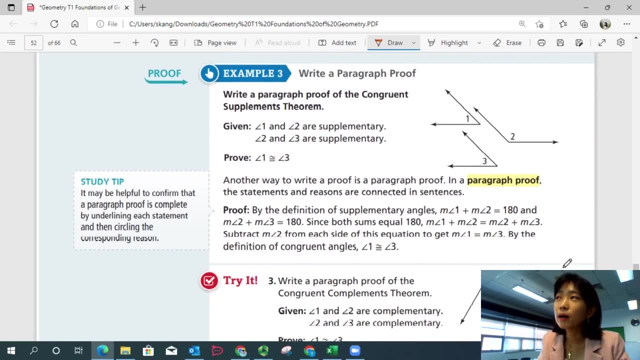 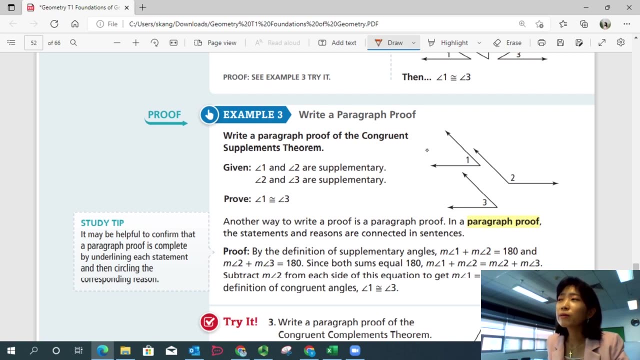 by definition of congruent angles. Let's prove that in example 3.. Write a paragraph proof. Write a paragraph proof Of the congruent supplement theorem. What is a paragraph proof? Paragraph proof is when you write all the statements and reasons connected in sentences. 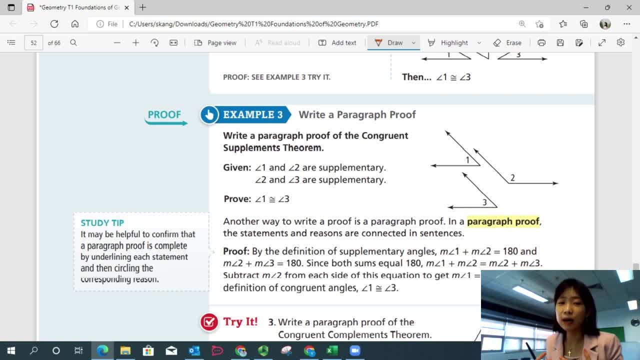 So it's like you're explaining it and you're writing down a big paragraph instead of columns, But you're basically writing down the same thing as the two column proof, but you have to write it in sentences. So if you prefer to write in sentences, 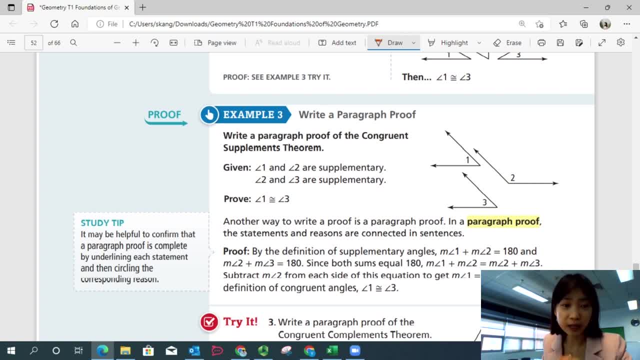 you will like paragraph proof much better than two column proofs. If you prefer to just write columns and then reason it out every time, then you will like two column proof, Okay, So let's look at how it's proven By the definition of supplementary angles. 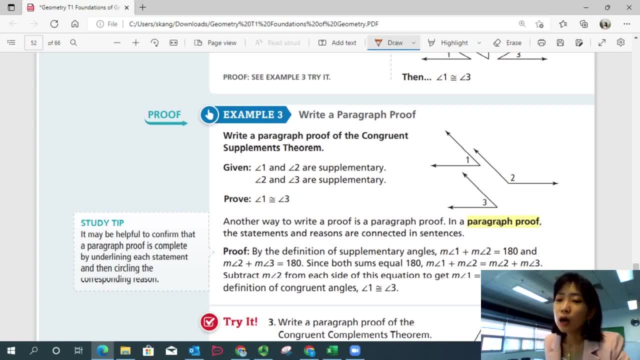 measure of angle 1 plus measure of angle 2 is equal to 180 degrees. Measure of angle 2 and 3 is equal to 180 degrees. since both sum equal 180 degrees. Measure of angle 1 plus measure of angle 2. 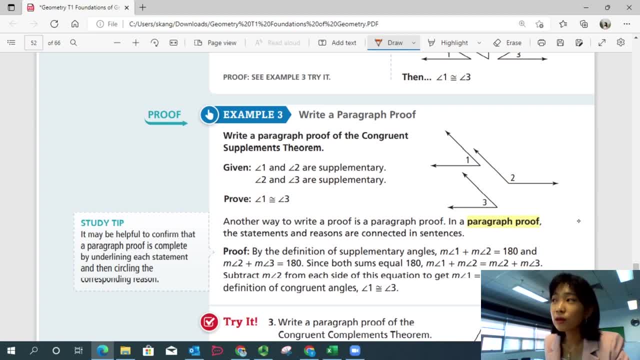 must equal to measure of angle 2 plus measure of angle 3.. And if you try to subtract both sides by measure of angle 2, then you get measure of angle 1 is equal to measure of angle 3.. So by the definition of congruent angles, 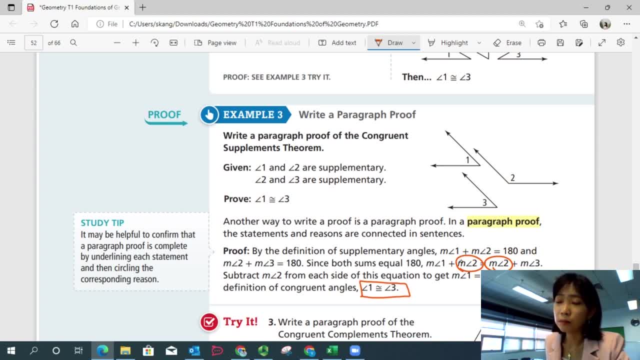 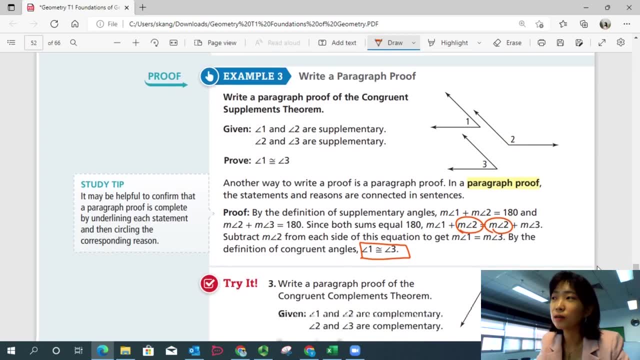 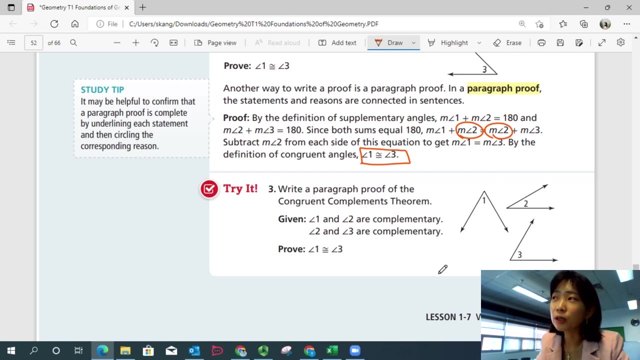 you can say that angles 1 and 3 are congruent. Now, using a very similar paragraph proof, you can prove theorem 1-3.. Write a paragraph proof of the congruent complements theorem, Given that 1 and 2 are complementary. 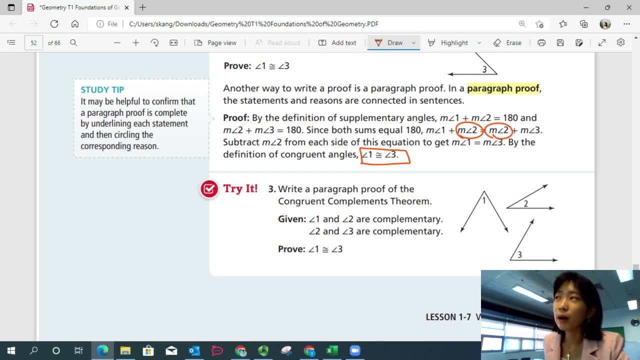 and 2 and 3 are complementary. write a paragraph proof. It could be very similar to that. See if you can do it by yourself. Come back when you're ready for answers. Okay, All right, Are you ready? How are you going to start? 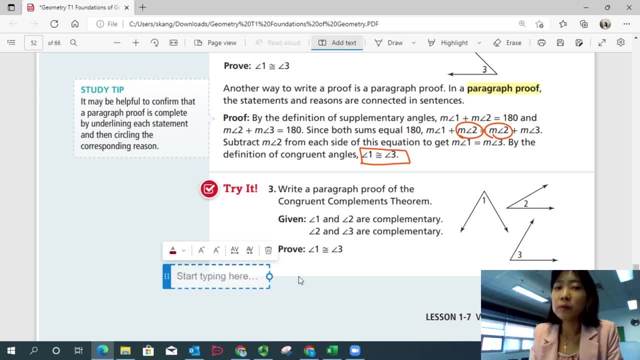 By the definition of supplementary. We don't have supplementary angles here, so we're going to start with the complementary angles. Yeah, by the definition of complementary angles, What do you know? Measure of angle 1 plus measure of angle 2 is equal to 90,. 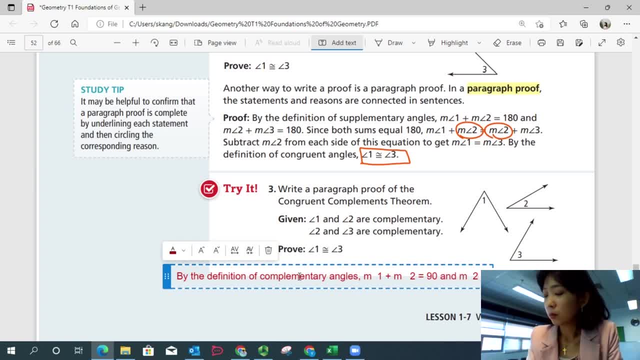 and measure of angle 2 plus measure of angle 3 is equal to 90.. I'm going to put angle in a moment. Okay, And then what? And then we can say we can set up an equation, just like we did, for example, 3.. 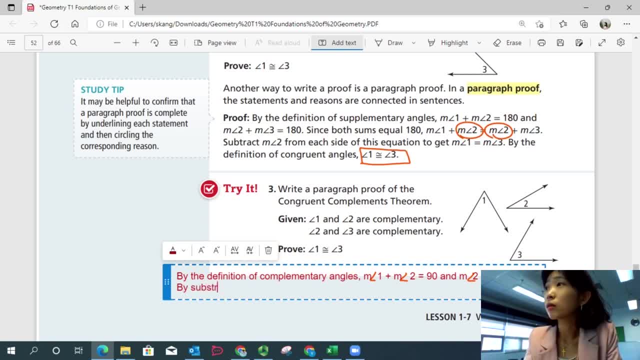 Right, So by substitution. substitution: measure of angle 1 plus measure of angle 2 is equal to measure of angle 2 and measure of angle 3.. Okay, And then what? And then you can subtract both sides by the same term. 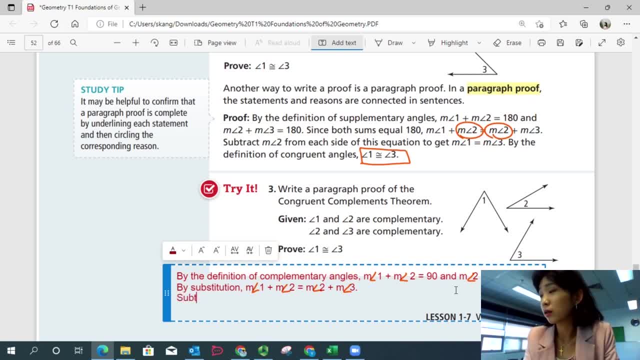 the measure of angle 2.. Subtract measure of angle 2 from each side to get what Measure of angle 1 is equal to measure of angle 3.. And by the definition, definition of congruent angles, your angle 1 is: 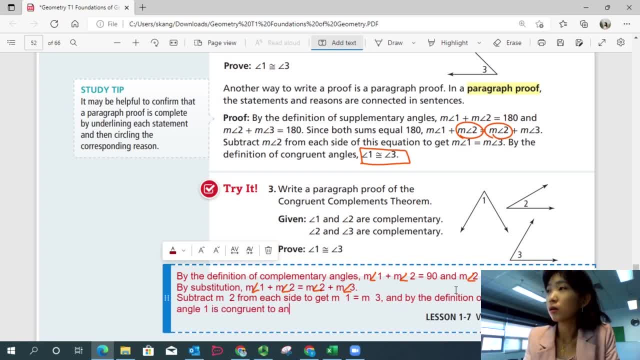 angle 1 is congruent to angle 3.. There you go. That was a paragraph proof. You just need to make them into sentences And that's it. Okay, Are we ready for more theorems and proving? Now we're just getting started. 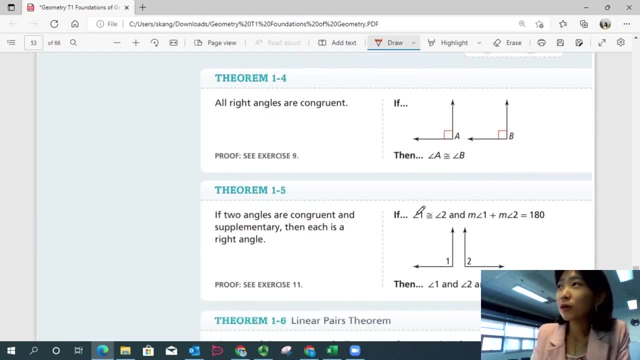 More practice. Let's get more practice. Alright, we get more theorems. Next page, Look at theorem 1-4.. All right, angles are congruent, Obviously, But this is a theorem. You have to prove it, Okay. 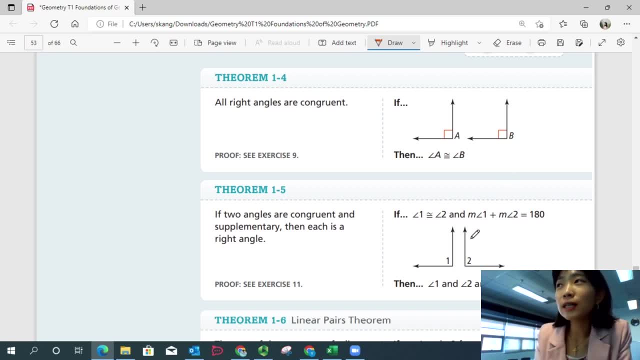 Theorem 1-5.. If two angles are congruent and supplementary, then each is a right angle. Now we're talking about right angles. Okay, If two angles are congruent and they are supplementary, they must be a right angle. 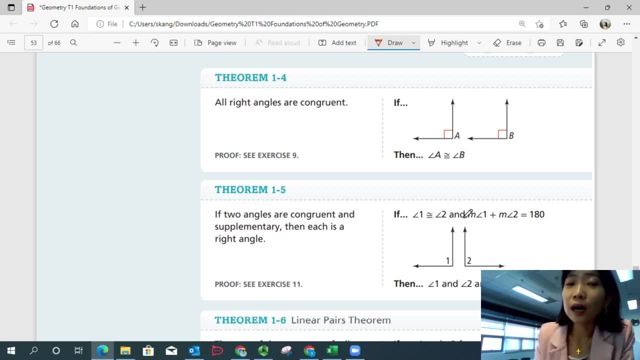 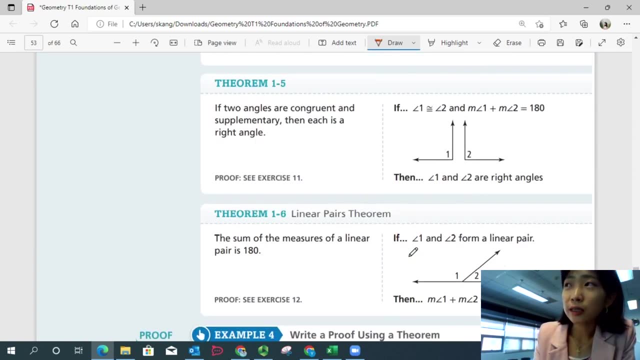 We're saying that there's no other angle that could be supplementary to each other and they're congruent. Alright, Theorem 1-6.. Linear pair theorem. Now, this theorem is very important. You're going to be able to use it. 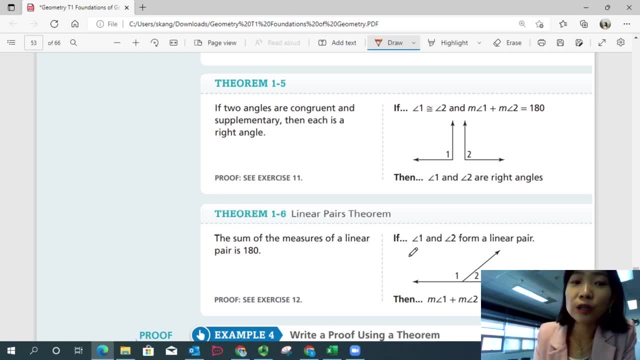 over and over again in future lessons. Look at what it says. The sum of the measures of a linear pair is 180 degrees. So if you have a linear pair, that means there's supplementary angle, And if you get a sum of that, 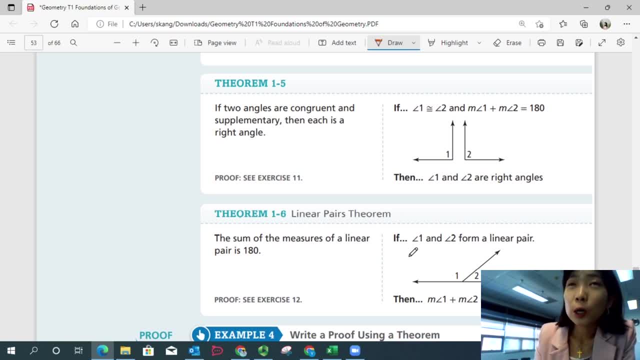 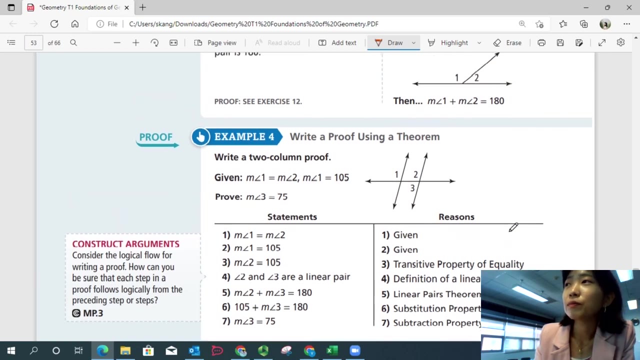 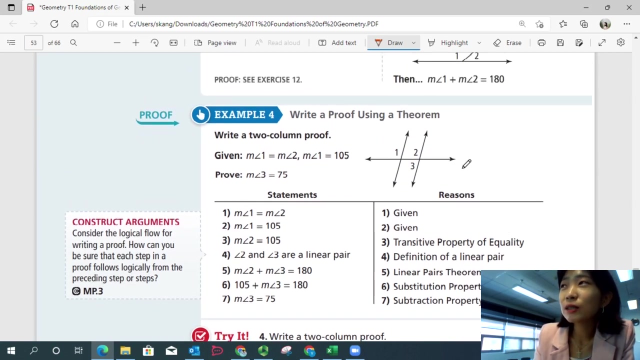 that's 180 degrees. You know that, but we're going to prove that in order to reason that out and prove other things. Okay, Example 4 is a proof of this. So let's write a two-column proof. Going back to a two-column proof, 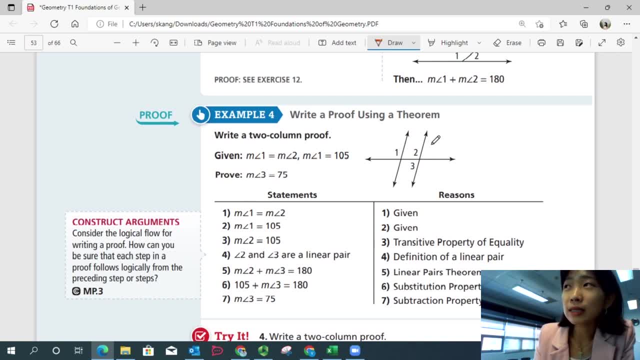 Given that measure of angle 1 and 2 are the same and measure of angle 1 is 105, okay, they're equal to each other. we're going to prove that measure of angle 3, which is supplementary to angle 2,. 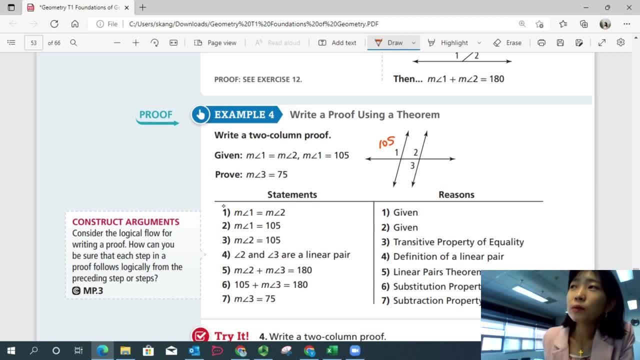 is 75.. So first we're going to state the given facts. Measure of angle 1 is equal to measure of angle 2, given. Measure of angle 1 is equal to 105, given, And that means measure of angle 2. 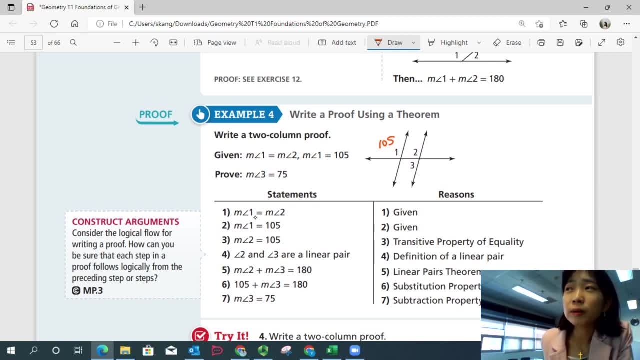 is 105 as well by transitive property of equality Right, A equals B, B equals C, then A equals C Transitive property, And so angle 2 and angle 3 are linear pair. definition of a linear pair. 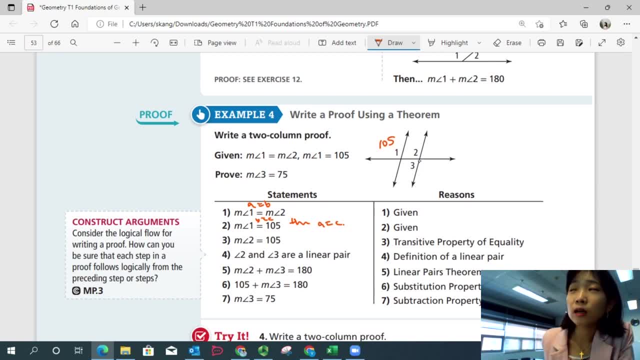 If they're on the same line and they're divided by a single ray or line, then they're a linear pair, Right, And that means their measures are going to add up to 180 degrees by a linear pair's theorem. So 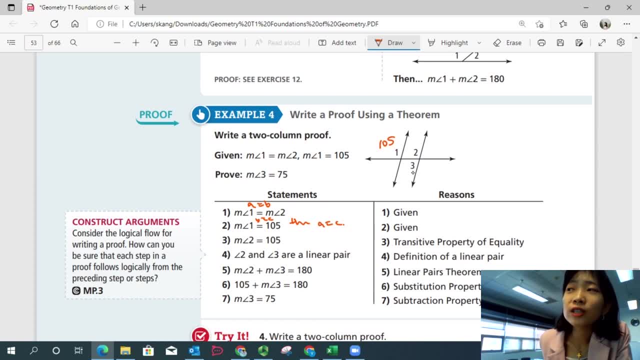 if you add 105 plus measure of angle 3, you should get 180 degrees by substituting this into this equation, because we know measure of angle 2 is 105.. Right Now we can solve for the equation and say measure of angle 3 is 75,. 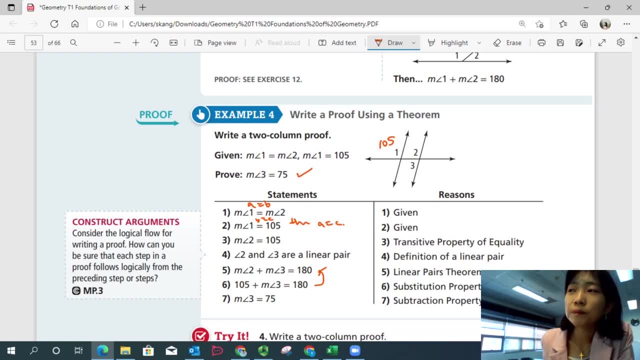 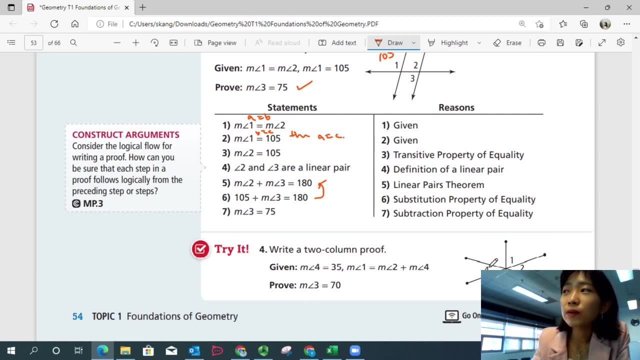 and that is all we need to prove what we need. Okay, Alright, try number 4.. Write a 2-column proof for the given fact that measure of angle 4 is 35, and 1 is equal to 2 plus 4.. 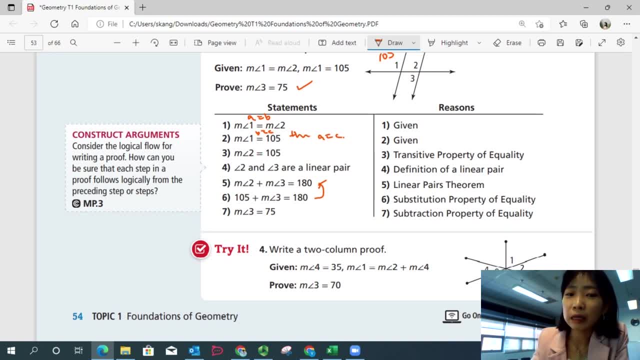 Using that, prove that measure of angle 3 is 70.. See if you can write your own 2-column proof. Make sure you state the given information first and then think about how you're going to get to that final statement in order to prove that. 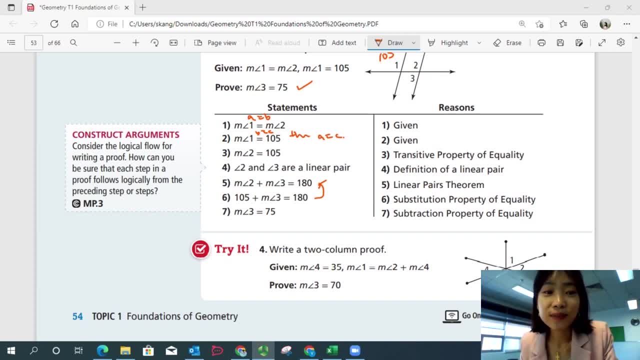 Okay, are you ready to check the answer? This is your last try-it for the lesson. Alright, let's look at the 2-column proof. We're going to write a statement section and then the reasons section, Right? So first, 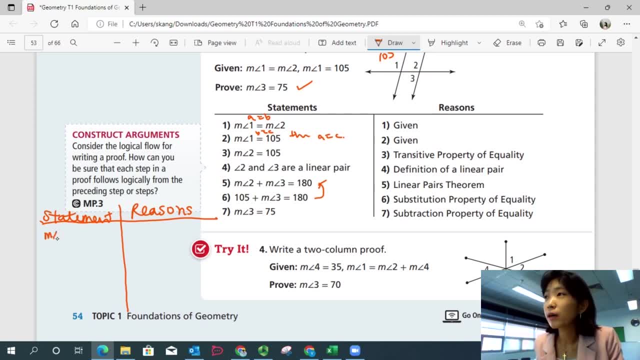 what do we have? The given statement, Measure of angle 4 is equal to 35. And using that, this is 35. We're going to use this information later. That measure of angle 1 is equal to 2 plus 4.. 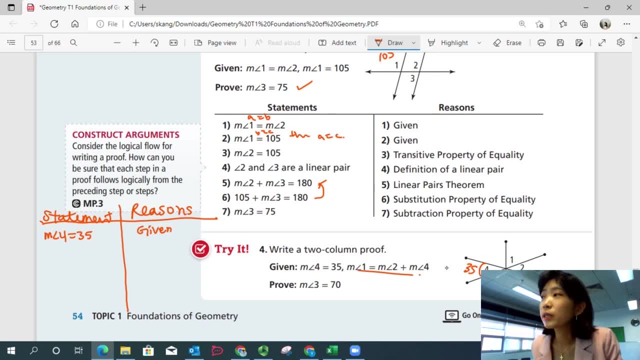 But right now, in order to use it, before we use that, what do we know? 4 and 2 are vertical angles, So that means 2 must also be 35. So let's state that as well. Angle 4 is congruent angle 2. 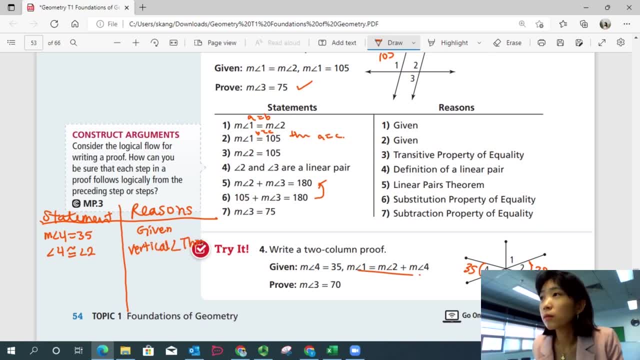 by vertical angles theorem And then say that the measure of angle 4 is equal to measure of angle 2.. Notice that when you're talking about measurement, you can write an equation, because we're dealing with numbers, But if you're talking about the angles, 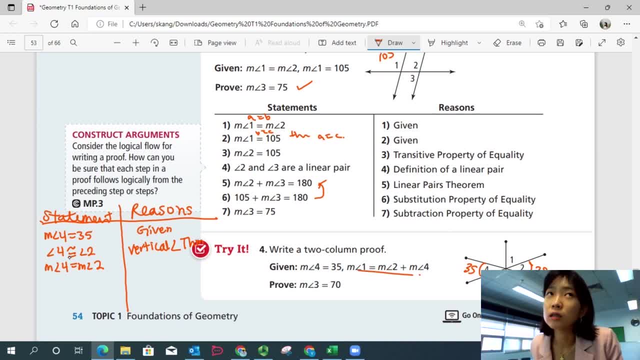 and lines and something that's not a measurement. we have to write them as a congruency statement or similarity statement- that we're going to learn later on. But we cannot just say they're equal to each other, They're congruent. Measure of angle 4 is equal to measure of angle 2. 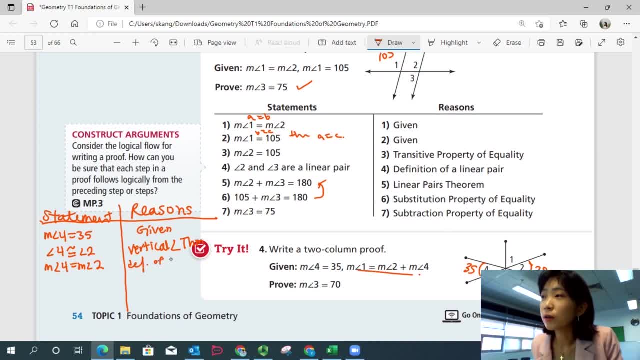 by definition Of congruent angles. Okay, And then that means measure of angle 2 is equal to 35 as well by transitive property of equality, And then use the given information: Measure of angle 1 is equal to measure of angle 2. 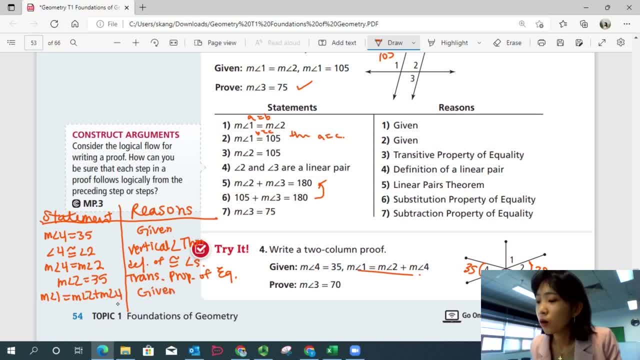 plus measure of angle 4 given. And what do we do? We know angles 2 and 4.. Right, So measure of angle 1 is equal to 35 plus 35. By what reason? Substitution? Because we already know that. 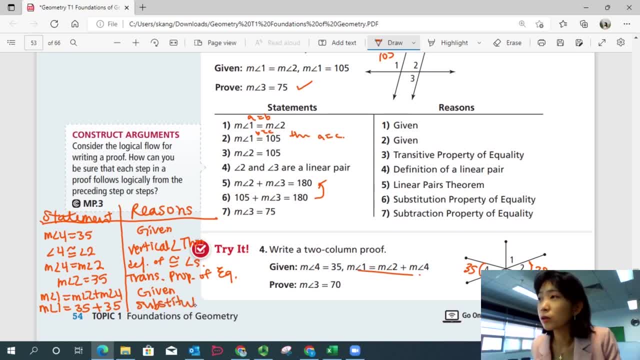 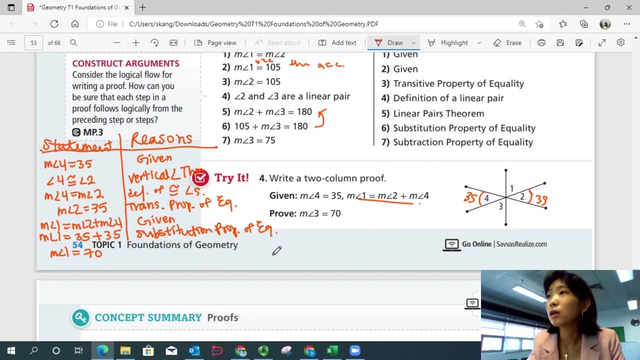 they both equal to 35.. Substitution: Property of equality. And then what? And then we just compute Right, So measure of angle 3 is equal to 70. And we can say that we simplified. And then what are we trying to prove? 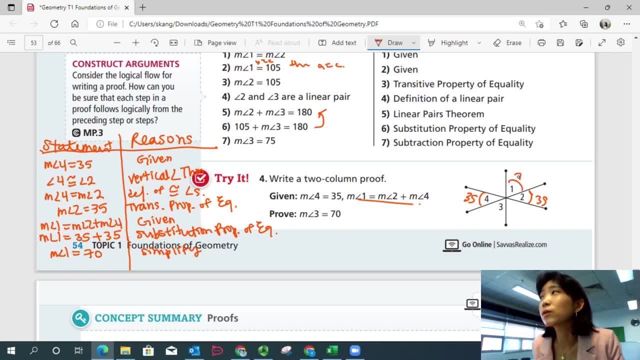 That measure of angle 3 is 70. Right Now, we just prove that this is 70. How can we prove that measure of angle 3 is 70 as well? They're vertical angles, Right. So measure of angle 1. 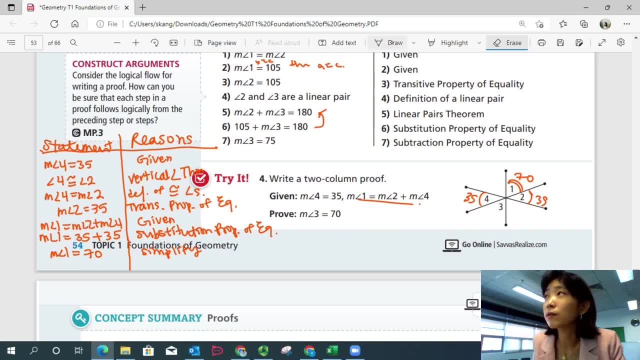 before we talk about measures, we have to state that they're vertical angles. So angle 1 is congruent to angle 3 by vertical angles theorem. And then we're going to continue here. That means measure of angle 1 is equal to measure of angle 3. 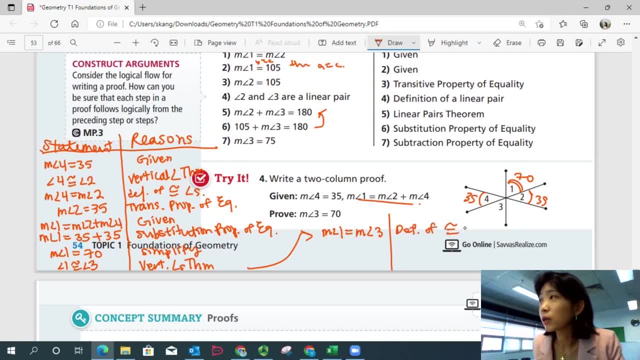 by definition of congruent angles. And finally we can say that measure of angle 3 is equal to 70 by transitive property of equality. Whew, It's just very tedious because you're listing them out one by one and it looks like a lot. 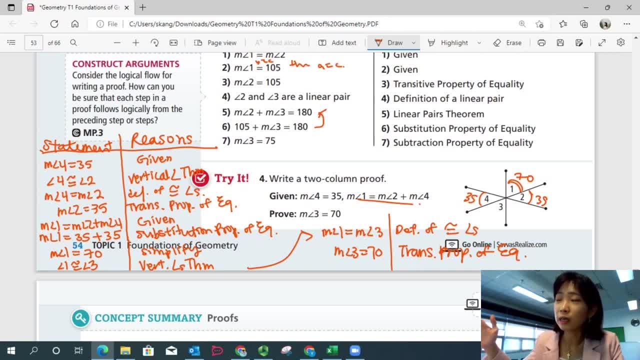 But you can actually think through this logical statement in just a few seconds. So that's your planning process. before you write a two-column proof, Before you write a proof, think about how you can prove it. You're going to hide the fact that measure of angle 3. 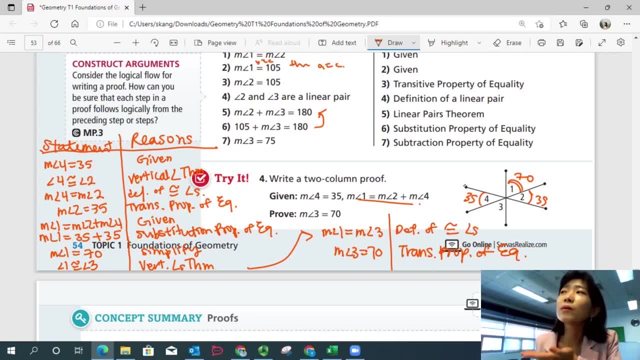 is going to be 70.. Try to figure it by yourself. Start with the given information. If that's 35,, then that should be 35. And if 1 is equal to 2 plus 4, then 1 must be 70.. 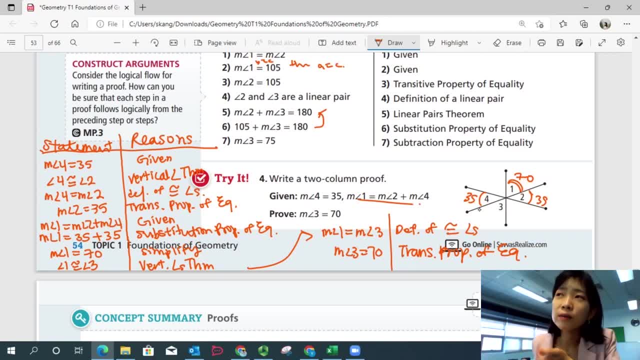 And if 1 is 70, then 3 must be 70 because of vertical angles, And you have solved it by yourself. Now you can write a two-column proof using the exact thought process that you have had in mind while solving it. 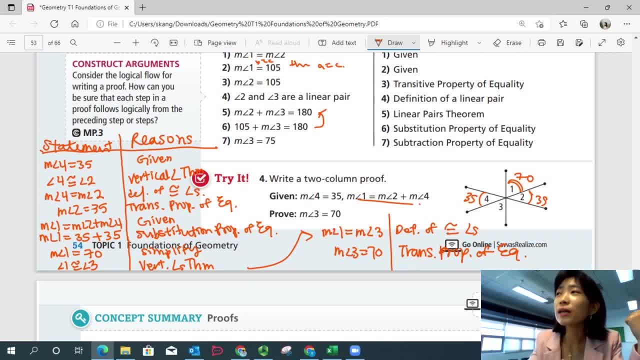 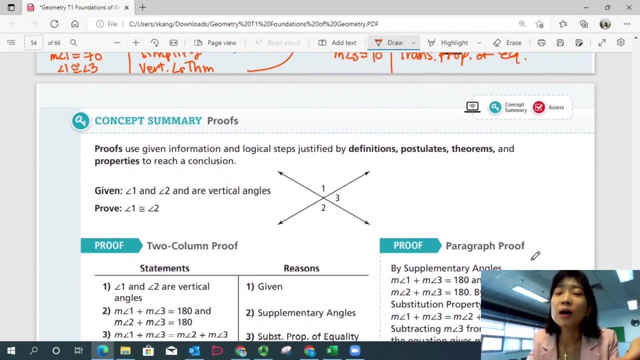 Does that make sense? I hope it does. Okay, so we are going to summarize our lesson. What did we learn in this lesson? A lot. We learned a lot about theorems, proofs, two-column proof, paragraph proof and some notations. right, 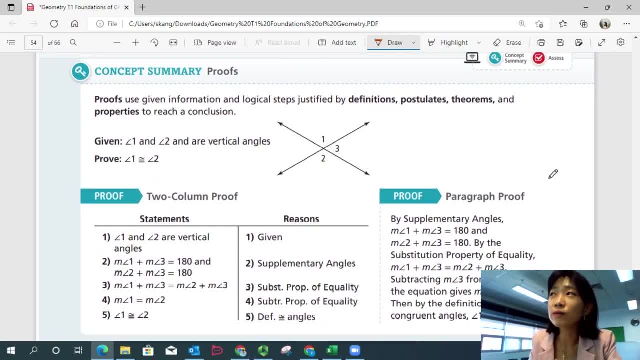 So proofs is given, information on logical steps justified by definitions, postulates, theorems and properties to reach a conclusion. It is part of a deductive reasoning and it is a strong reasoning skill. So, for another example, if you're given that angle is 1. 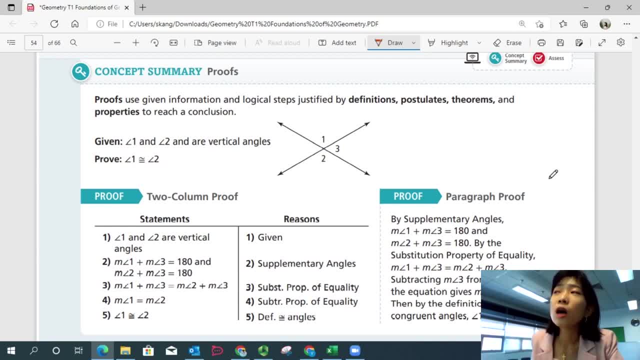 into your vertical angle and you want to prove that they're congruent. you can write the proof in two different ways: two-column proof, paragraph proof. There are numerous other ways to write proofs, but these are the two proofs that we learned today.